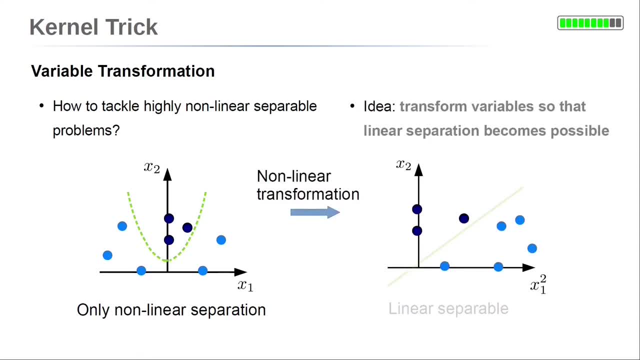 by a parabolic boundary. So if we use a quadratic transformation of, for example, the input variable x1, we obtain the result displayed on the right side. Now this problem is linear separable and we can use a support vector machine for classification. Consequently, variable transformations will help us to apply support vector machines more. 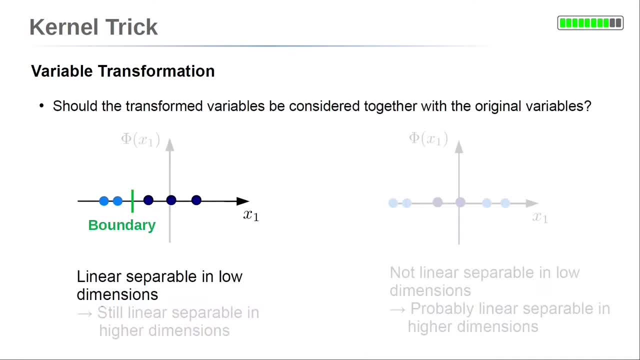 generally, You might wonder if it is beneficial to consider the original variables in addition to the transformed variables. Here we will look at a very simple example to clarify this. We consider a single independent variable, x1, only On the left side The two classes, the light blue and the dark blue dots, are clearly separable by a linear 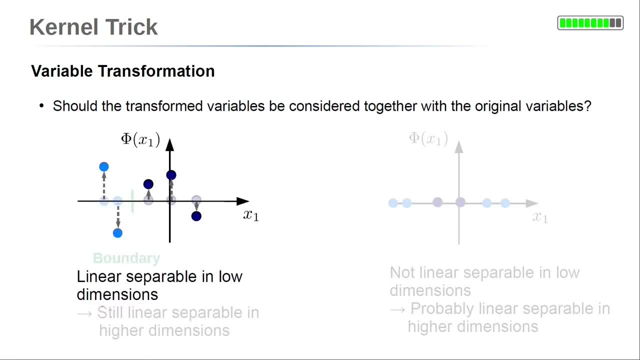 boundary. Now we apply an arbitrary variable transformation phi of x. This shifts the data points around. However, we still can separate the two classes by a linear boundary. The reason is because the classes cannot mix with respect to their position. The variables can shift their position to the x1 axis. 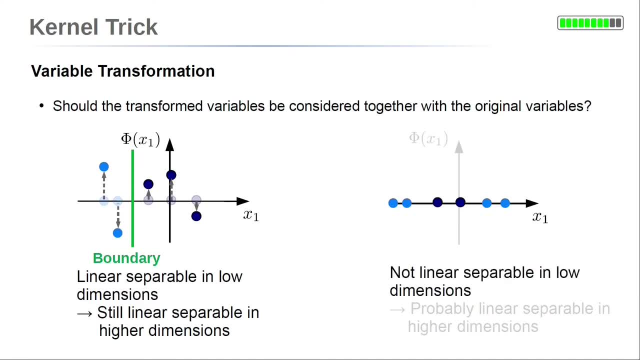 Next we take a look on the right side. In this example, the classes are not linear separable. Again, we can apply a variable transformation. A good transformation now allows for separation, But even if not, it is no disadvantage to incorporate the original variables. 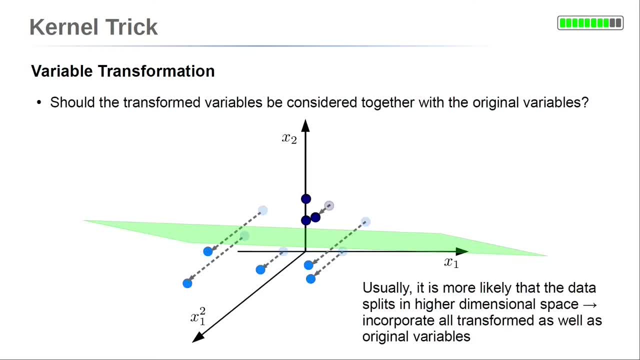 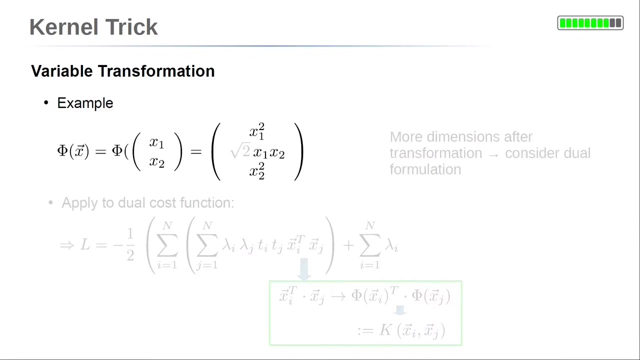 In total. usually it is more likely that the data splits in higher dimensional spaces. So to incorporate all transformed as well as the original variables is very beneficial. So let's consider a concrete example. We have two dimensions with input variables x1 and x2.. 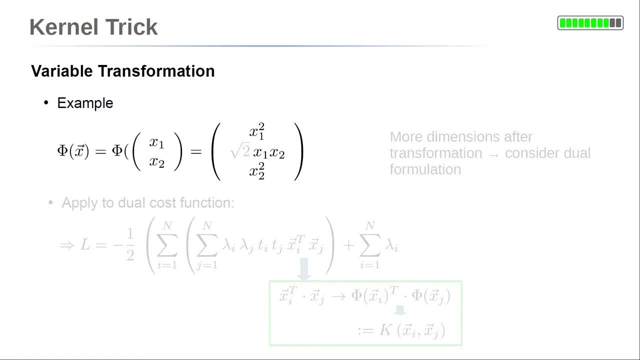 We want to perform a variable transformation to all possible second order terms. These are x1 squared, x2 squared and x1 times x2.. Here we put a factor of square root of 2 in front of the term x1 times x2.. 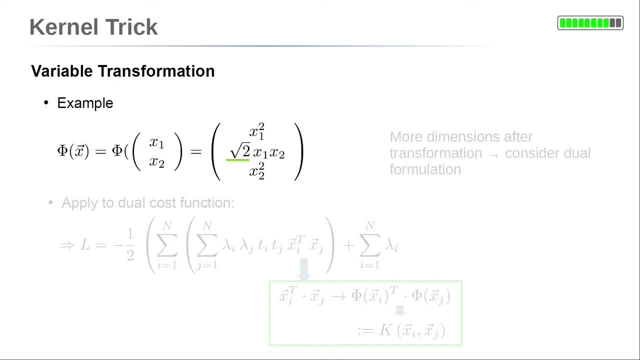 This is for convenience, as we will see later. If we want to take these three transformed variables In addition to our original two variables into account, We have in total five variables. So variable transformations can produce a lot of extra dimensions. This is why the dual formulation with the Lagrangian cost function is so useful. 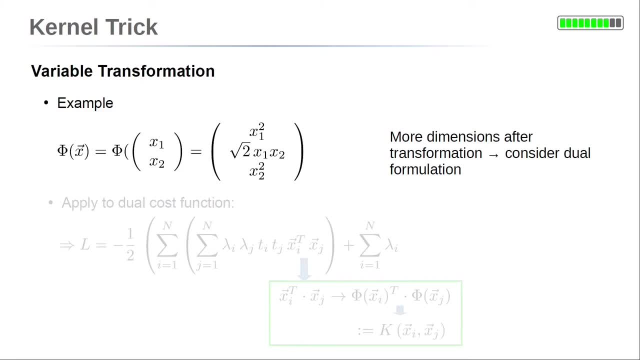 For this cost function the computational efforts, independent of the number of dimensions considered. But the question is How to incorporate the variable transformation easily into the Lagrangian cost function. The variable transformation affects the dot product of vector x i times vector x j. 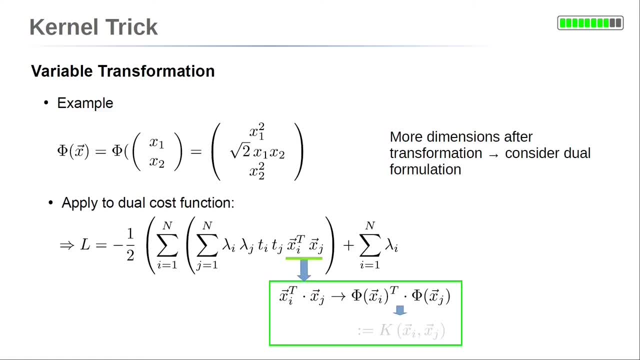 To apply the variable transformation is straightforward. First, it is applied on the vector x i. Second, it is applied on the vector x- j. Then, Calculating the dot product of x i times x- j, The result is the dot product of the transformed vectors. 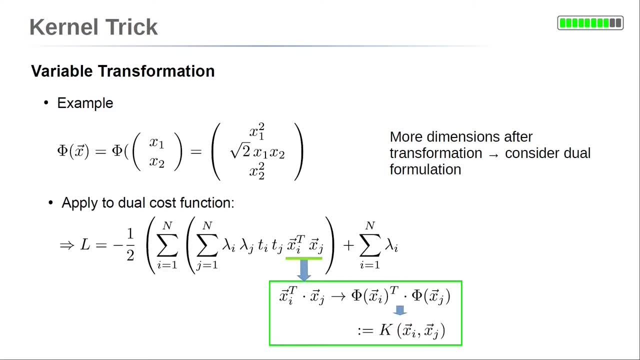 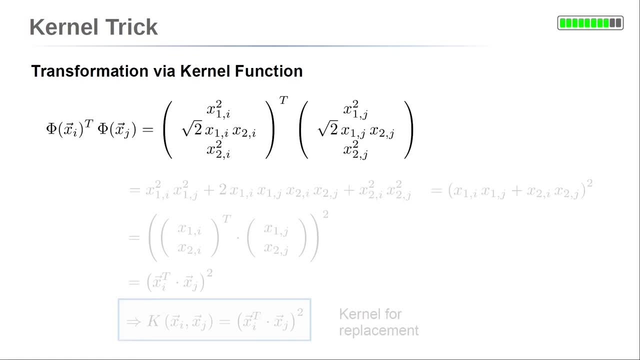 This result is denoted by capital K, The so called kernel function of the transformation. We will calculate the corresponding kernel function for our example. So we transform the vector x i and the vector x j individually. This gives these two vectors with now three components each. 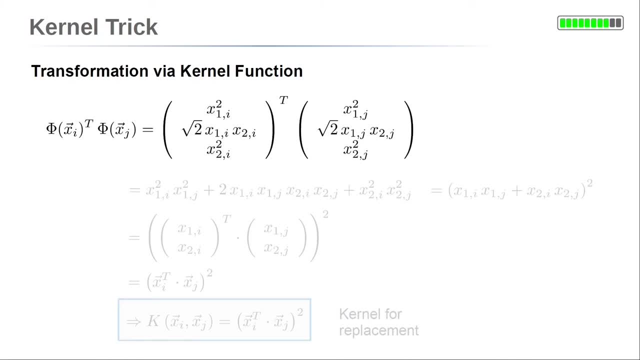 And in the following we will derive a different representation for the product of these vectors. The result is the following: Multiplying the product out gives X1i squared times x1j squared, Plus 2 times x1i times x1j times x2i times x2j. 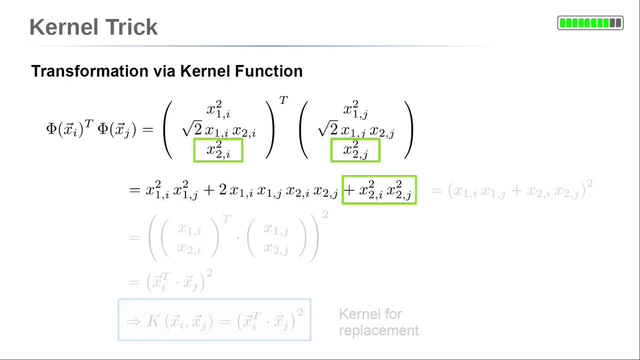 Plus x2i squared times x2j squared, Plus x2i squared times x2j squared, This will be x1j times x2j. Note that the multiplication of the two factor square root of 2 gives the factor of 2 in. 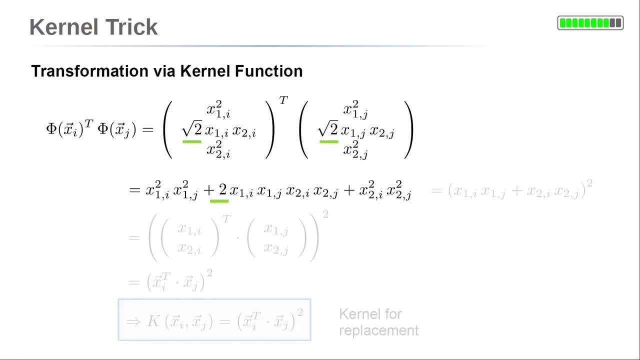 the term in the middle. This was the reason to incorporate this factor, Because now we can rewrite this as quadratic expression: The squared of x1i times x1j plus x2i times x2j. In this expression we have the vector components of xi and xj. 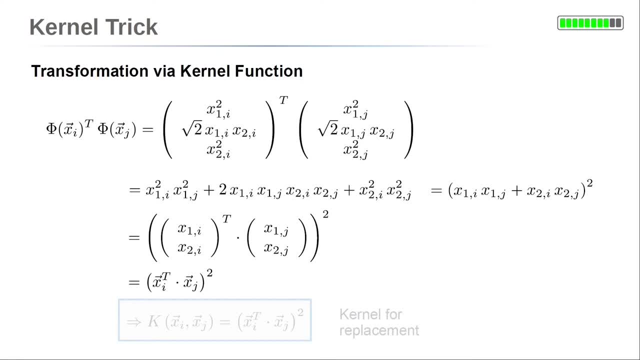 So in short notation, this is the squared dot product of vector xi times vector xj. This gives our final representation of the transformed variable product. So we can replace the product of vector xi and vector xj just by the squared of this dot product. 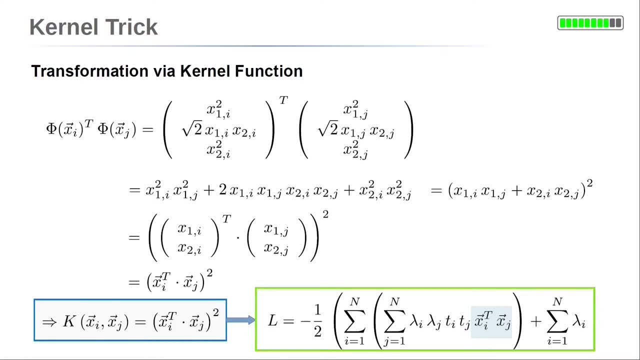 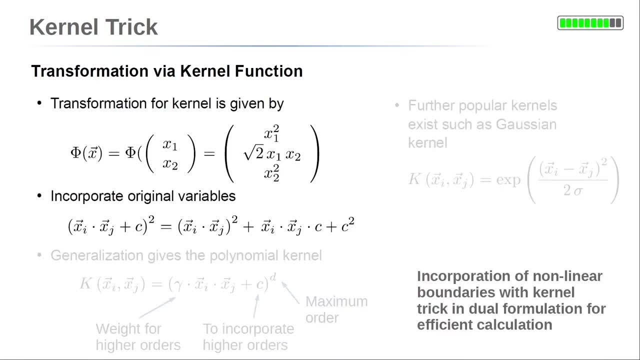 This incorporates our quadratic variable transformation. So far, we replaced our original variables x1 and x2 by three new variables: x1 squared, x2 squared and x1 times x2.. But what about our original variables x1 and x2?? What about our original variables x1 and x2?? 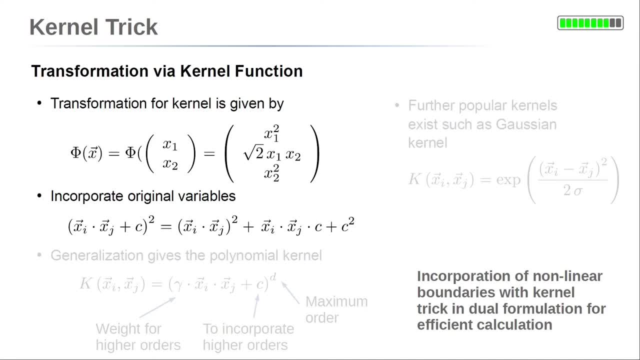 What about our original variables x1 and x2? How can they be incorporated? additionally, This can be done by adding a constant c to the dot product before calculating the square of it. We can multiply this out and see that we've incorporated the squared term for the transformed 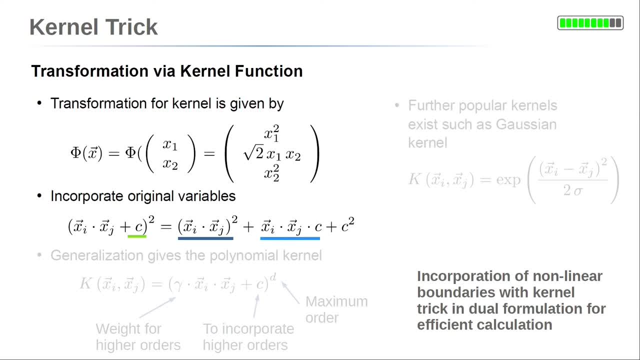 dot product And in addition we have the simple dot product of vector xi and vector xj. Let's begin with the original variable transformation of our original variable. This can be generalized to incorporate higher orders of variable transformations. The polynomial kernel replaces the square by an arbitrary order denoted by d.